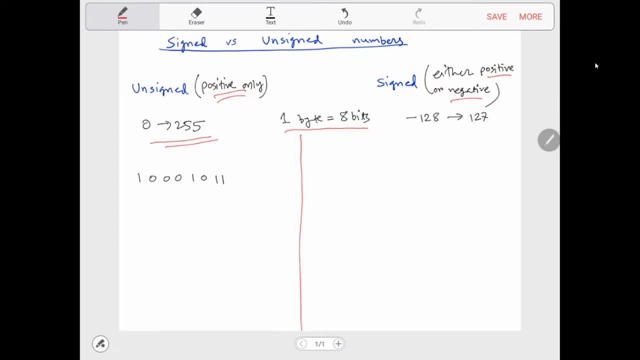 If the number is signed with 8 bits, you have a range between negative 128 to 127. Let's go over this example Now. remember it has to be mentioned whether a number is signed or unsigned. Let's say this is an unsigned number, So the positions are 0, 1, 2, 3, 4, 5, 6, 7.. 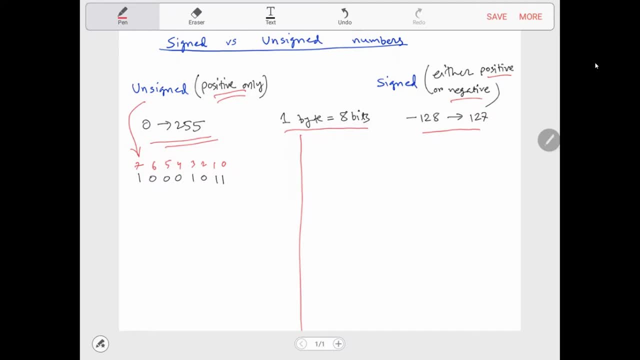 So the numbers in red are just the position of each binary bit. Let's convert this to base 10.. So you have 2 to the power 0 plus 2 to the power 1 plus 2 to the power 3 plus 2 to the power 7.. 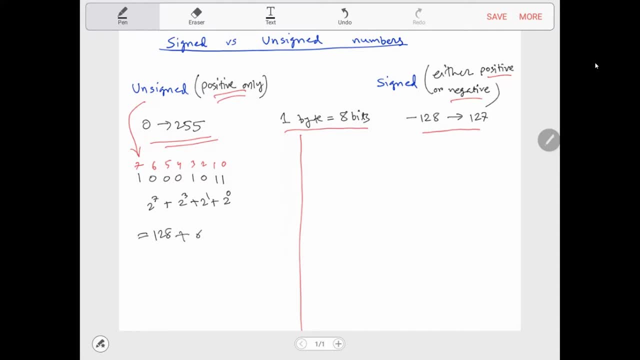 This gives you 128 plus 8 plus 2 plus 1.. if you add all this up, you get 139 in base 10. now let's do an example for a signed number. so here you have a signed number in 8 bits. remember for a signed number the. 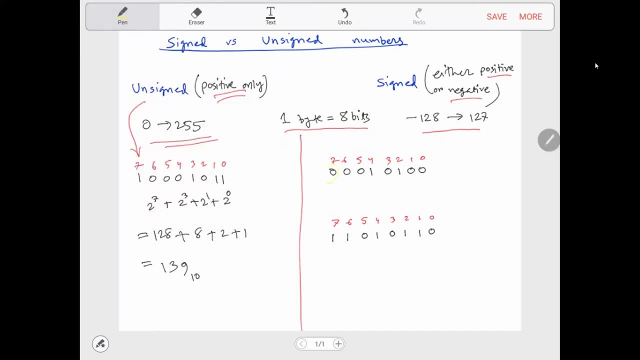 leftmost bit is the sign bit, so 0 means positive and 1 means negative sign. so let's convert this to base 10. this is pretty simple, you have. you have 2 squared plus 2 to the power 4 and this gives you 20 base 10. since this, 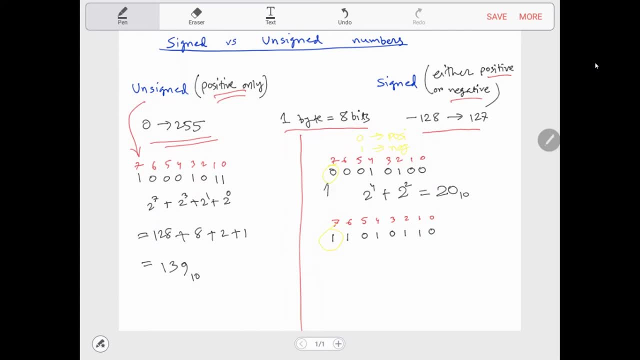 leftmost bit is 0. we know our number is positive. let's do the second one. so here you have 2 to the power 1 plus 2 squared, plus 2 to the power 4, plus 2 to the power 6. now this one, the leftmost bit. since it's a 1, you have a.